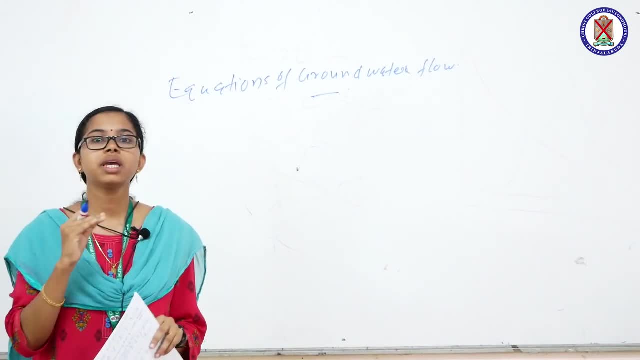 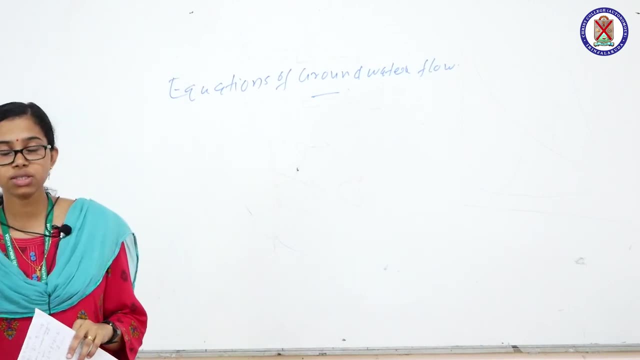 be four type of flow conditions, such as: there may be isotropic and homogeneous flow equations are there. anisotropic and heterogeneous flow equations are there, as well as anisotropic, homogenous flow equations are there, as well as anisotropic and heterogeneous flow equations are there. 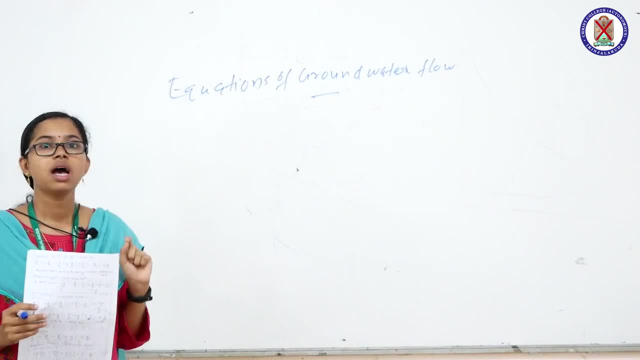 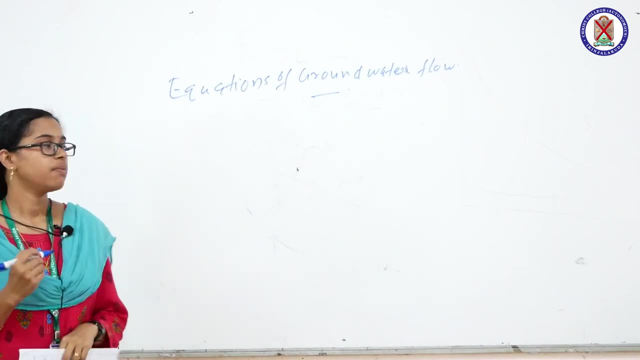 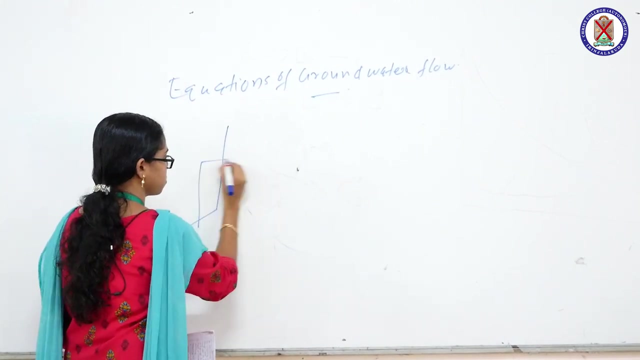 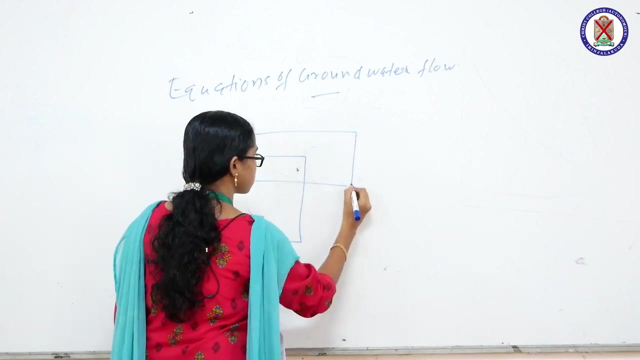 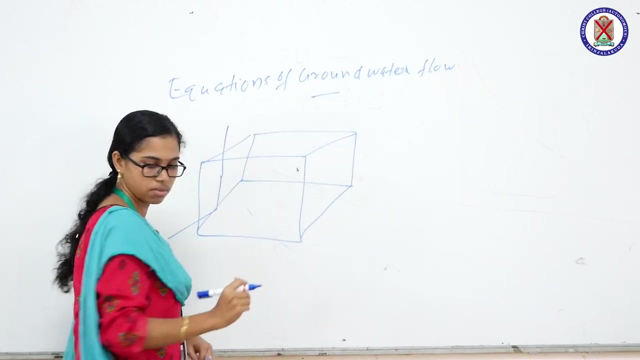 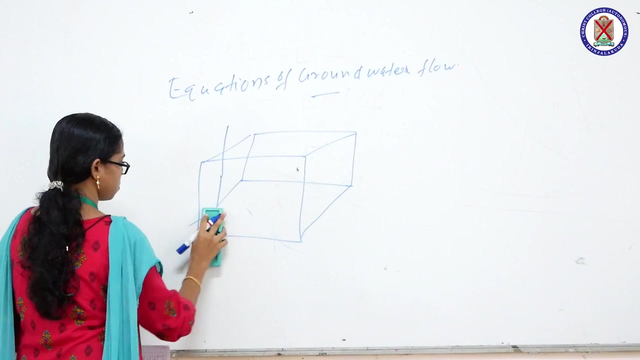 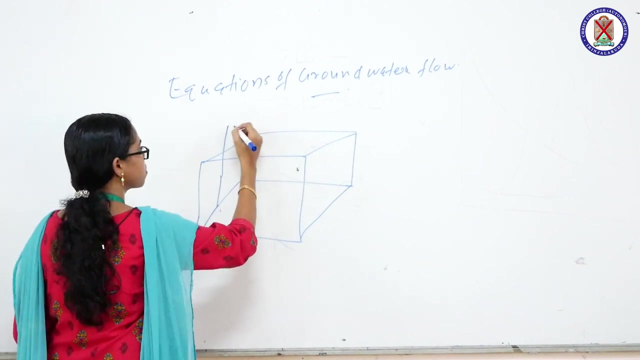 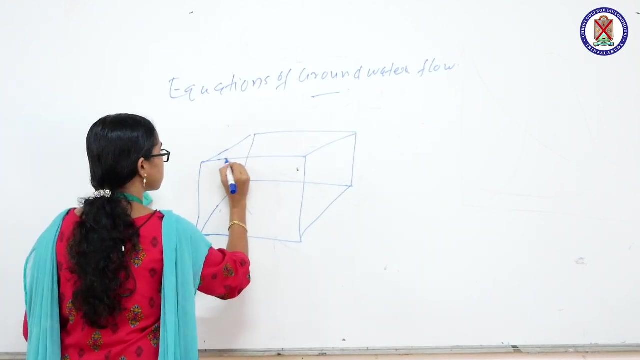 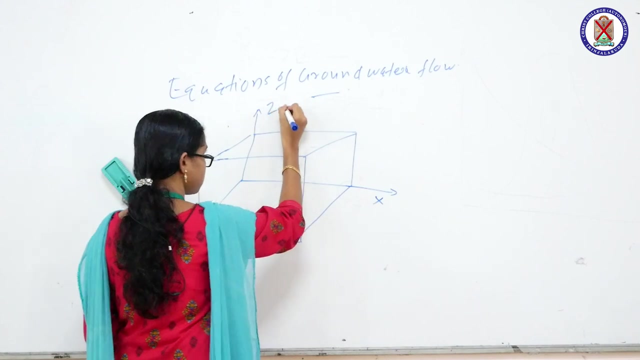 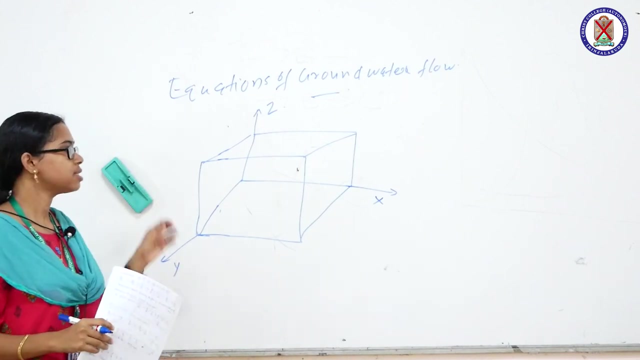 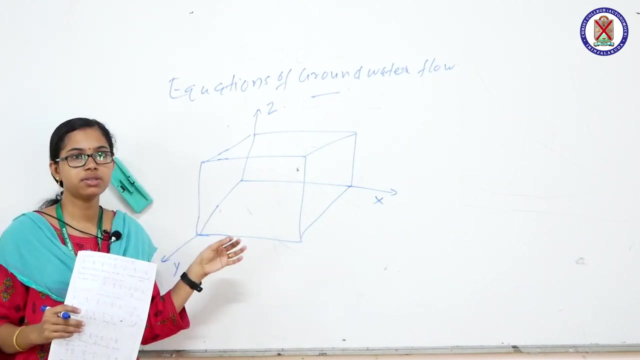 So here we are considering the aquifer as an anisotropic as well as a heterogeneous, Hence the flow equation will be. So, before we are going into the equation of particular ground water flow, let us consider an aquifer with a controlled volume, which means the volume will be controlled or specified. 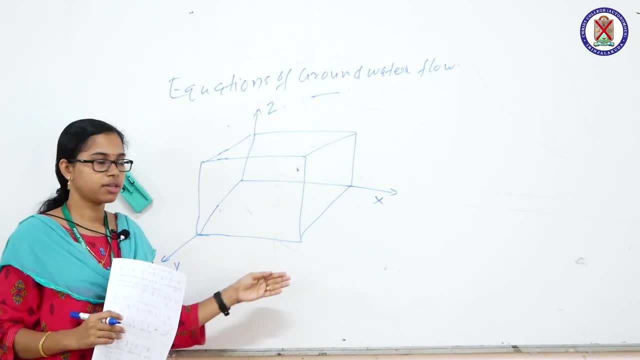 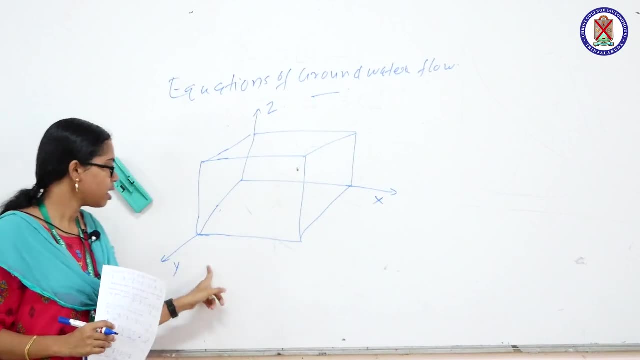 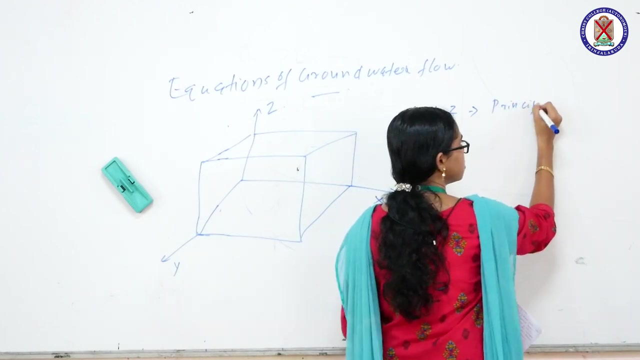 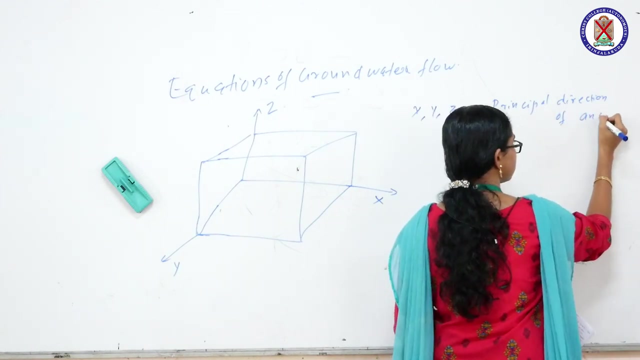 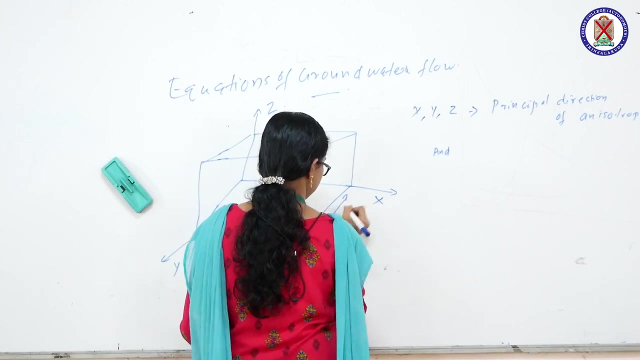 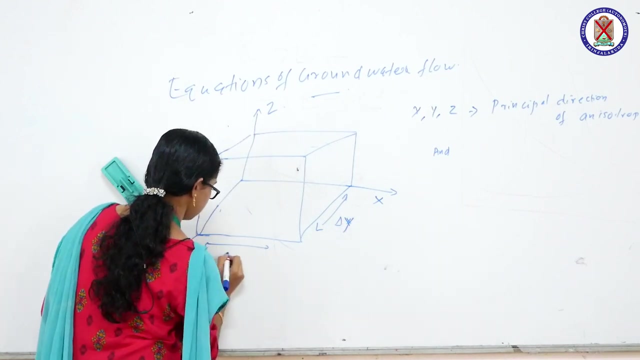 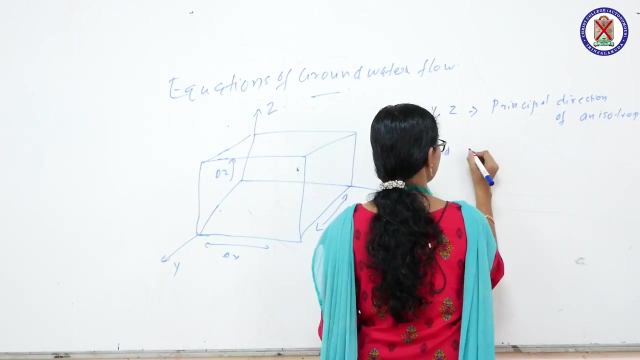 and we are considering an anisotropic aquifer. So this is an anisotropic aquifer and the x, y and z, that is, x, y and z, are the principal direction of principle direction, direction of anisotropy and delta and delta x, delta y and delta z represents. 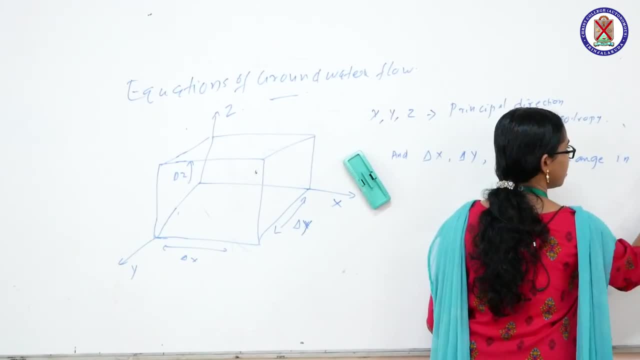 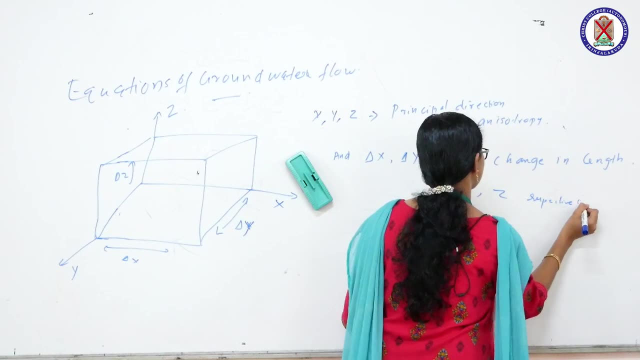 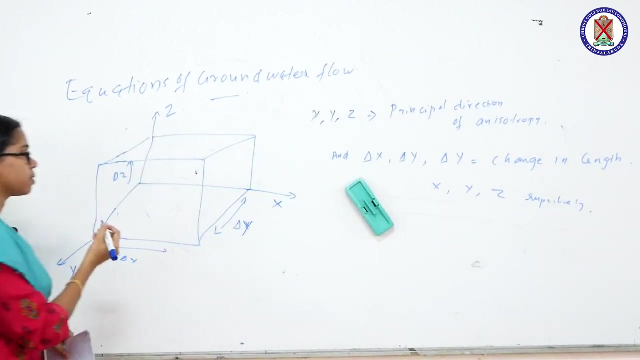 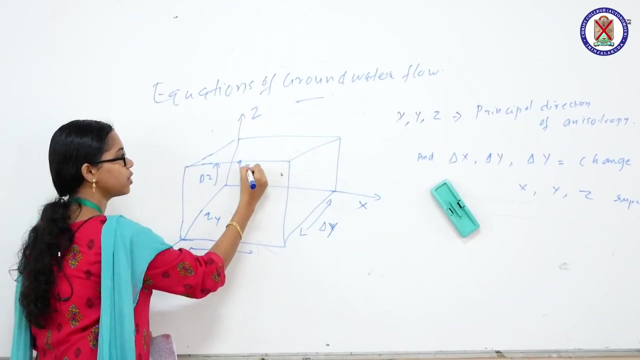 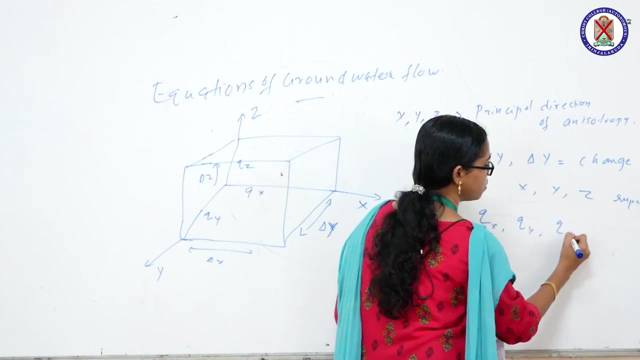 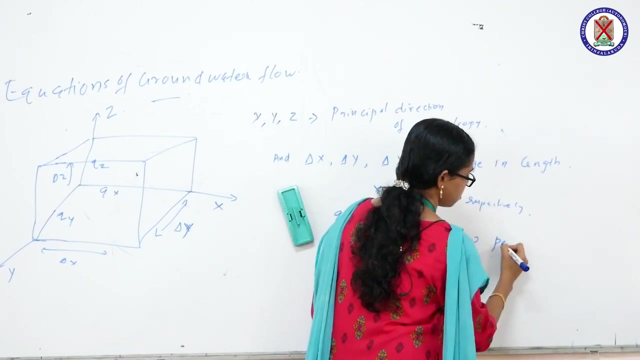 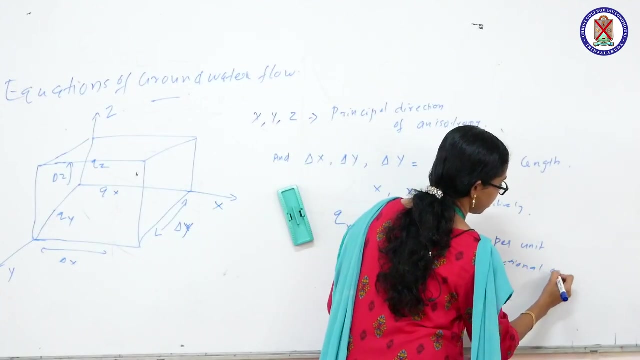 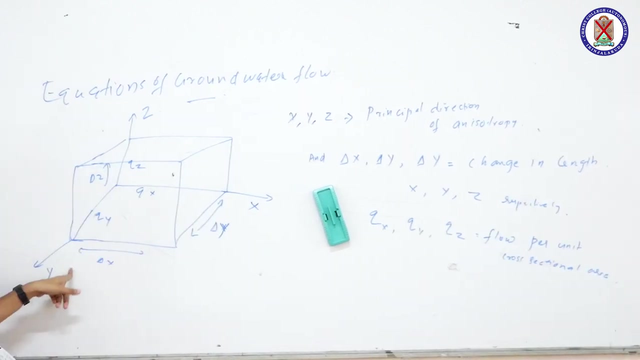 the change in length in the direction x, y and z respectively, and the q, the qx and qy and qz, which represents qx, qy and qz, represent the flow per unit cross sectional area, flow per unit cross sectional area. So this: x, y and z are the principal directions of anisotropy, and delta y, delta z and delta x. 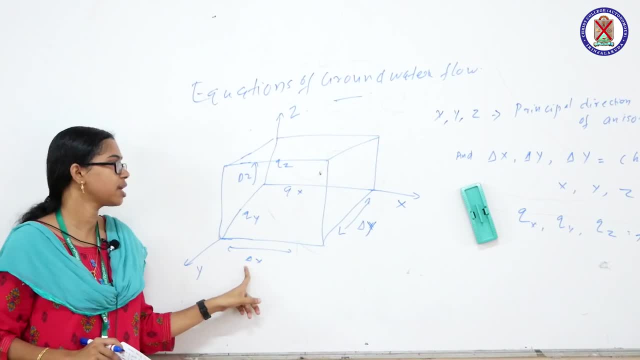 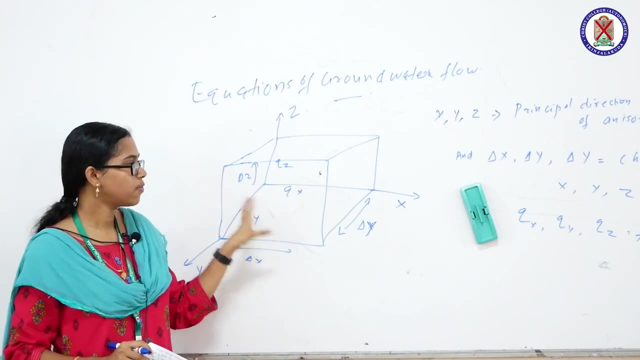 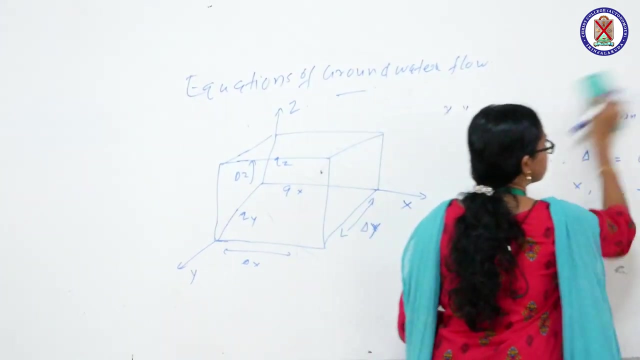 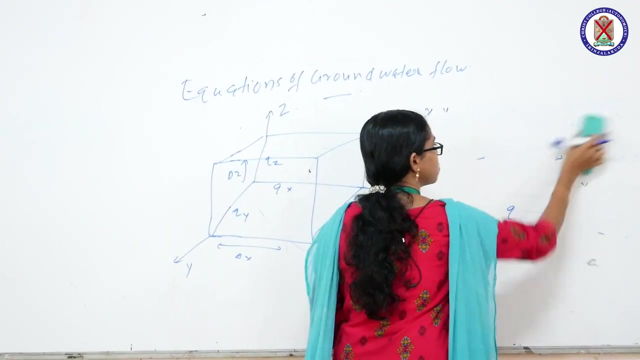 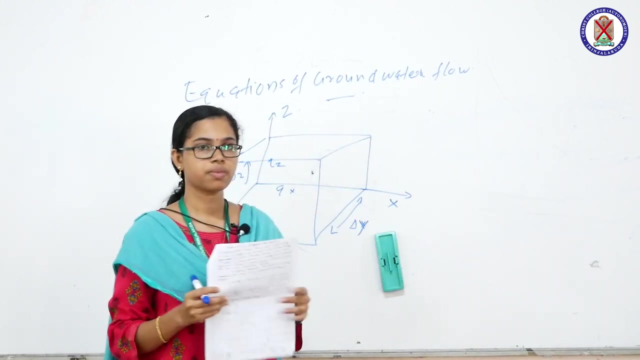 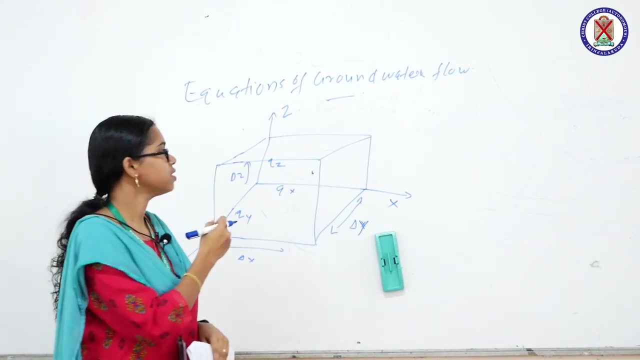 represent the change in length length with respect to the x and y z axis, x, y and z axis, and qx, qy and qz represents the flow per unit or discharge per unit cross-sectional area. So let us move to the flow equation or let us move to the derivation of particular flow. 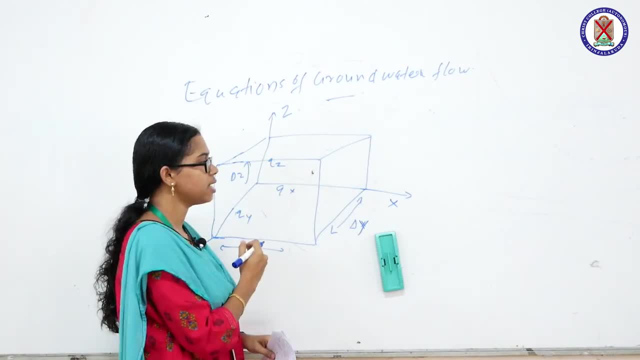 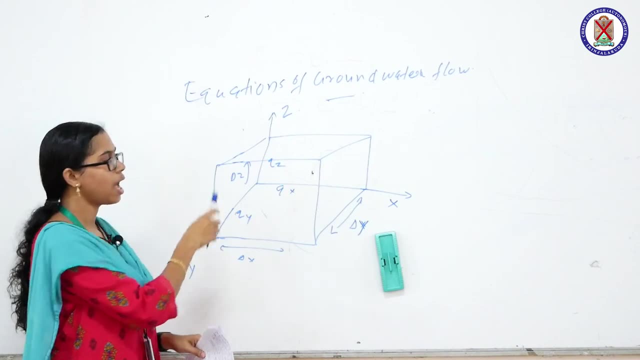 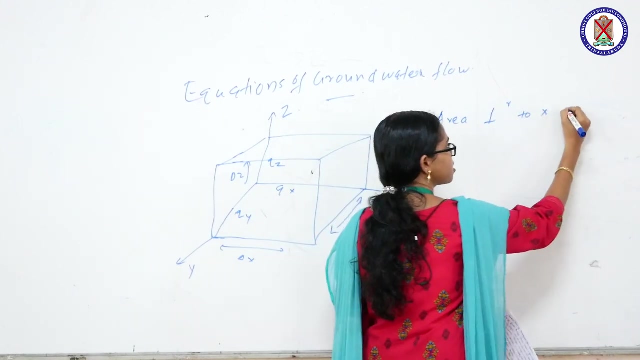 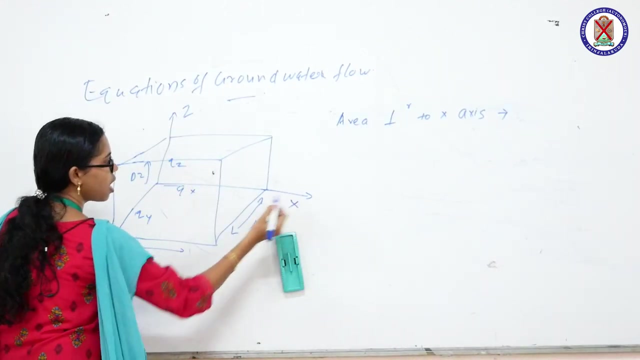 equation. So first of all we have to consider the area of area perpendicular to the x, y and z direction. So the area which are perpendicular to x axis is: so the area perpendicular to the x principal direction will be area of this particular particular flow. So let us 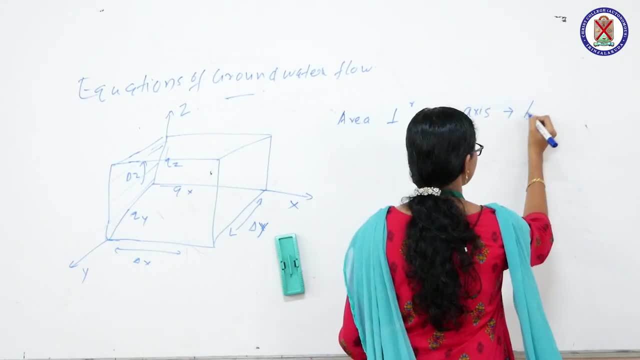 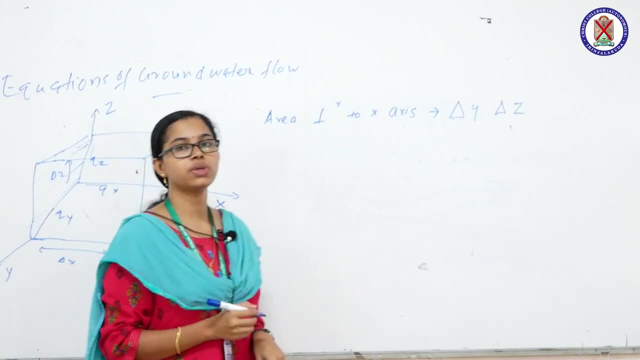 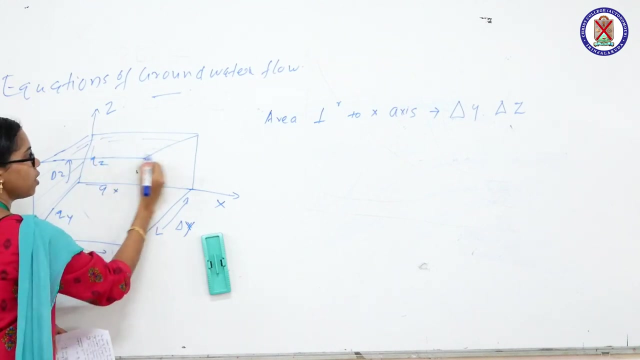 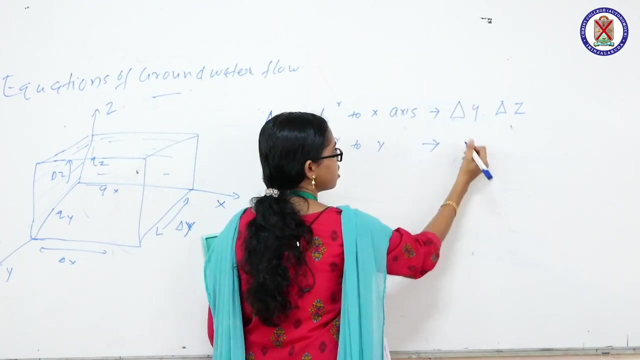 calculate delta x, which is equal to delta y, into delta z And the area perpendicular to the y axis. the area perpendicular to the y axis will be the area of this side, So we will get: the area perpendicular to y axis is equal to delta x into delta z, And.